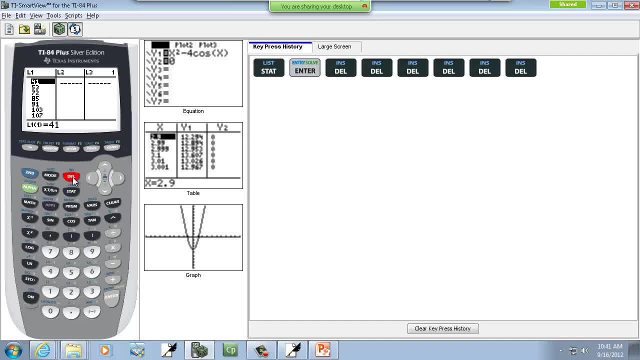 You can press delete over and over to clear those out. A lot of numbers in there. I was going for the safe way of clearing those out. I didn't realize I'd have to press delete a thousand times. Okay, and we'll put in our numbers. 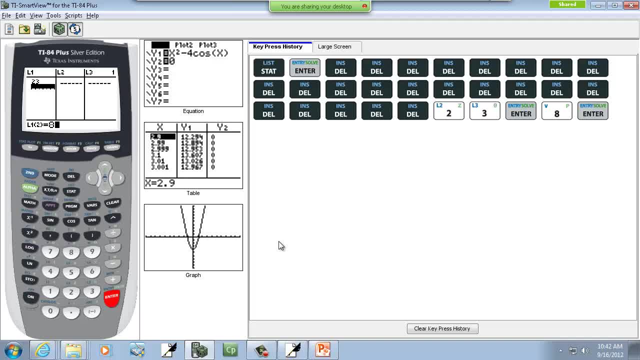 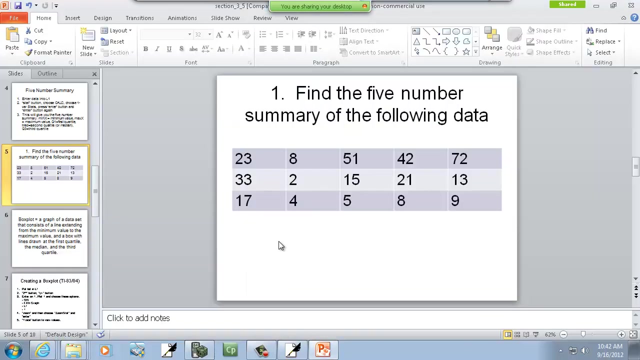 23,, so 23. enter 8. enter 51. enter 42. enter 72. enter 33. enter 2. enter 15. enter 21. enter 13. enter 17. enter 4. enter 5. enter 8. enter 9 enter. 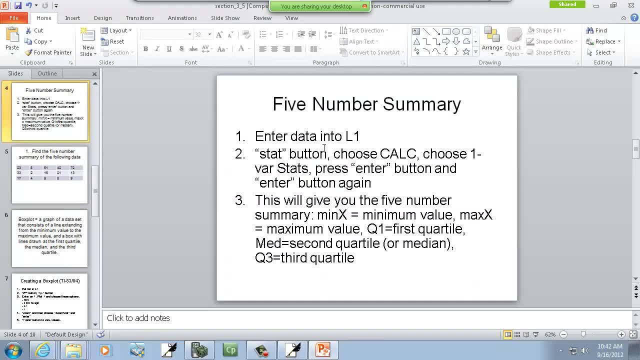 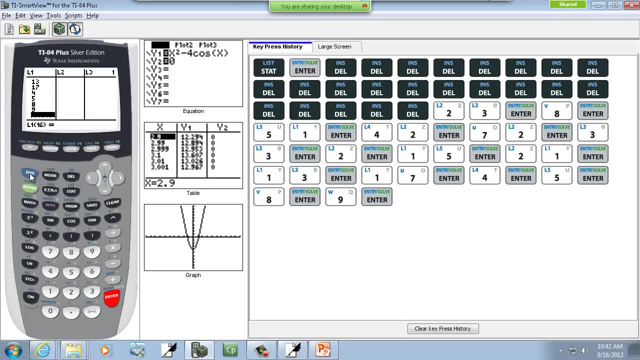 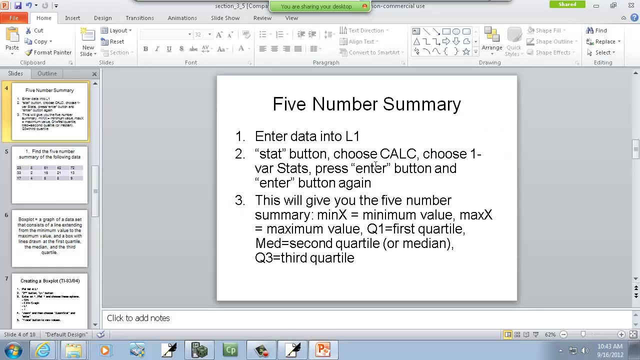 Okay, now over here I say: enter data into one. it's implied, any time you get your data input in, go ahead and exit out. So you do a second mode to exit out. Okay, then step two. it says stat button: choose calc, choose one of our stats, press enter and press enter again. 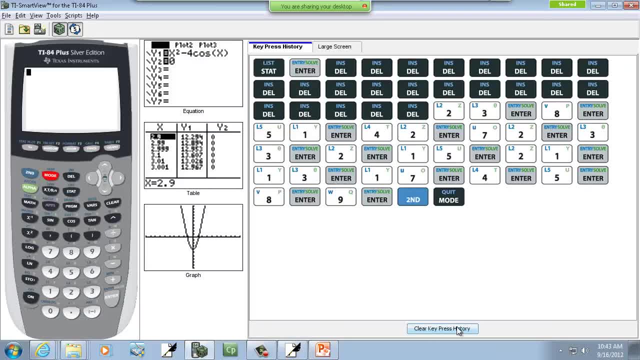 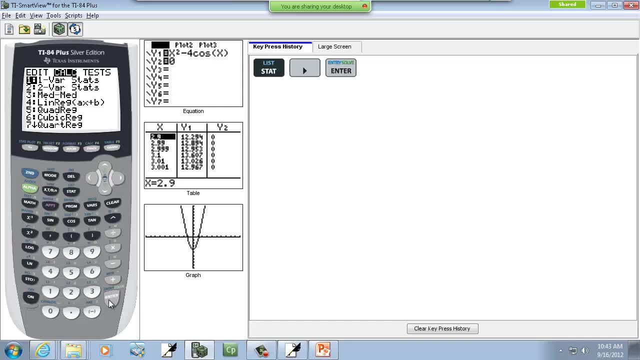 So we'll press our- let me clear that out- Press our stat button, right arrow to calc, and one of our stats is already selected. So we'll press enter on that And then we'll press enter again. Now it assumes that you put your numbers in L1.. So if you put them somewhere else, then you have to put in whatever list when you do the one of our stats. 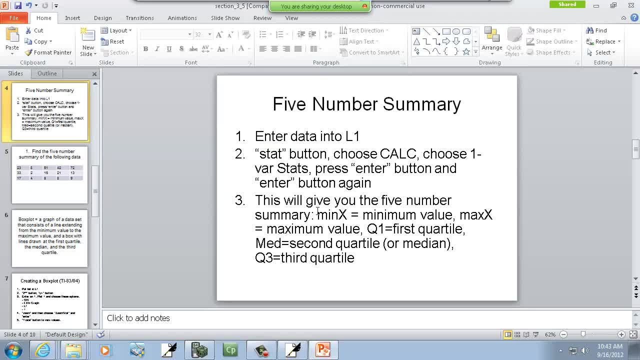 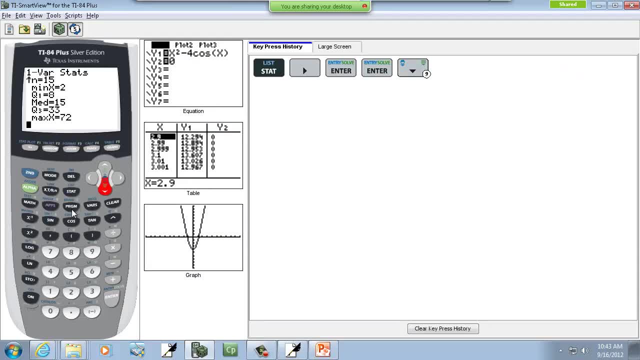 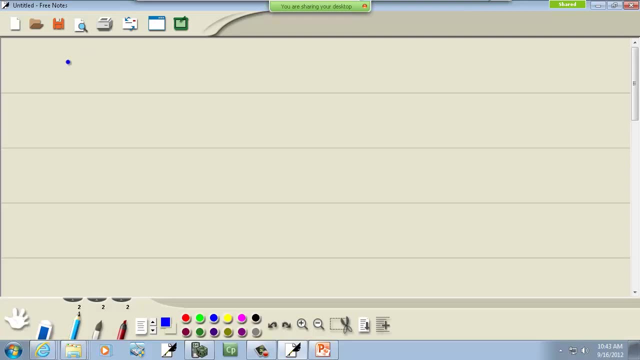 Now this doesn't tell you, but it says this will give you the five number summary and how to get that. So the first is your down arrow And the last five numbers are your five number summary. So let me write those down. So for our first example, we have 2,, 8,, 15,, 33,, 72.. 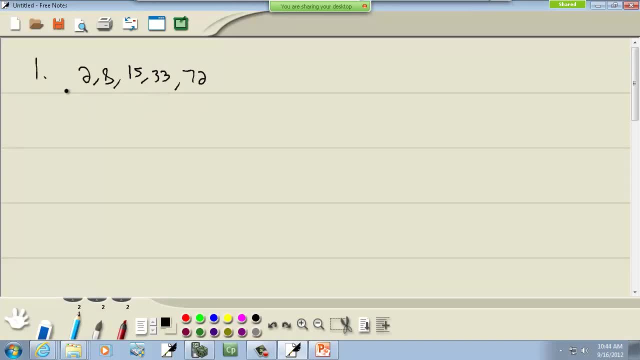 Now, you typically don't have to label these, So if I ask you to find a five number summary, it's always this order: This is a min, this is a max, this is Q1,, this is Q2, and this is Q3.. And Q2 is also your median. 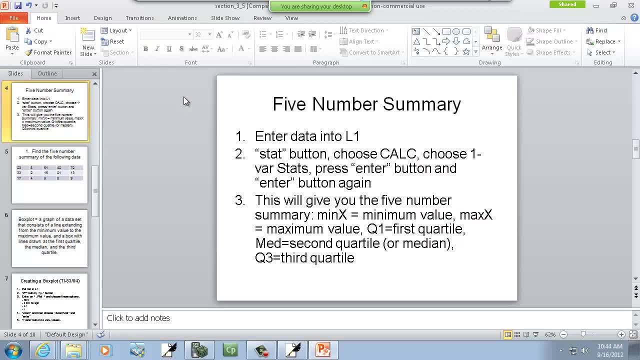 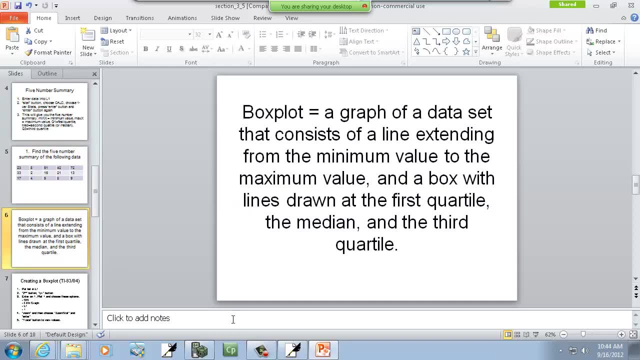 Tell you what. that's our five number summary, And this tells you this: what each one is. Okay now, box plot. This is a graph of a data set that consists of a line Extending from the minimum value to the maximum value. 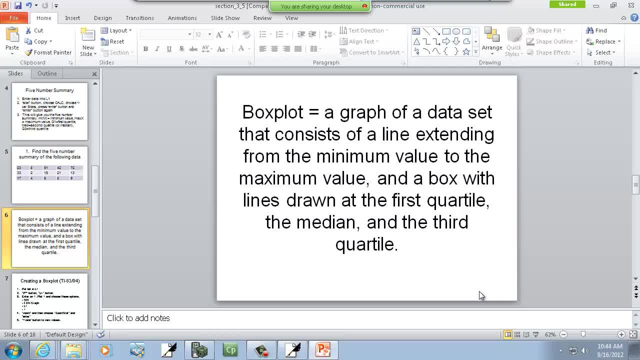 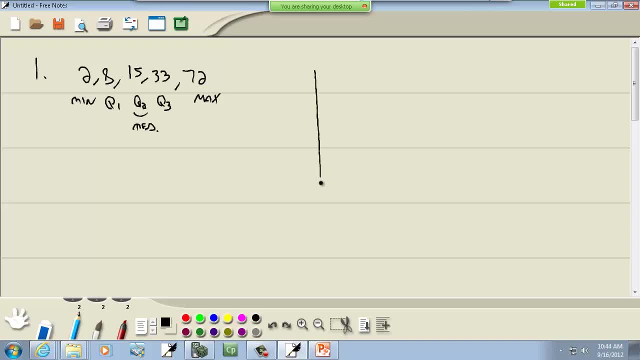 And a box of lines drawn to the first quartile, the median and the third quartile. Let me create a box plot based upon this data. Just to show it Now, our largest number is 72.. So I'm going to come over here. if I was doing this by hand, then I'm just going to put like 80.. 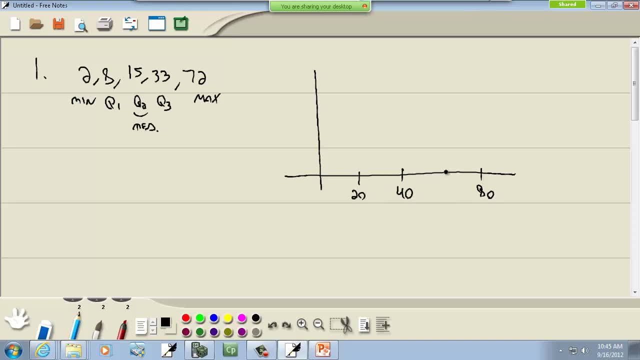 I want to choose a number I can easily divide by 2. And that would be 20. And this would be 60. And here would be 10. And this would be 30. Okay, so our min is 2.. 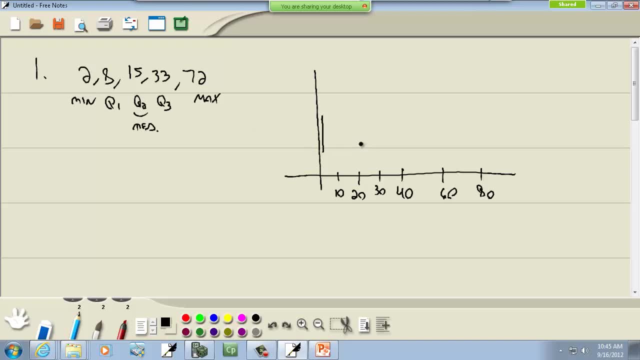 So I come here and I'll put a vertical line at 2.. Our max is 72.. Here would be 70.. So 72, maybe right there Nose should be the same height. And then Q1,, 8, we'll put a smaller vertical line. 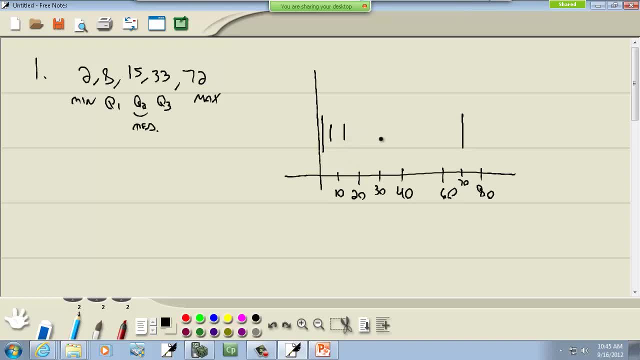 15, we put another smaller vertical line, And at Q3, 33, we put another one Like that, And then you draw a box like this around Q1,, Q2, and Q3. And then you draw a horizontal line going out to the min and max, like that: 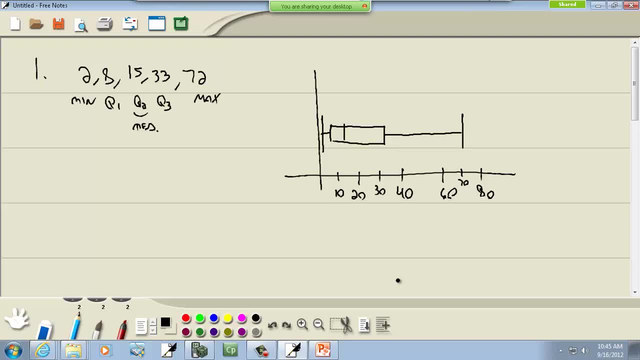 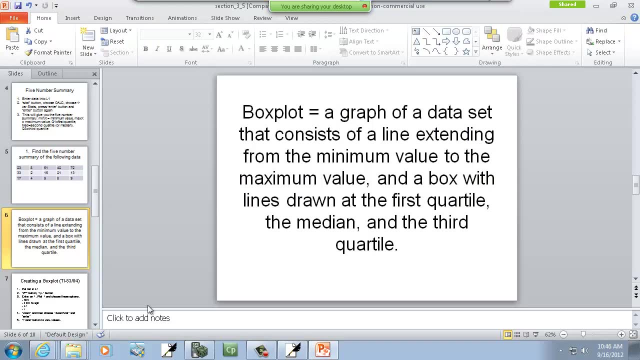 And that would be our box, plot by hand. They're not hard, Just get a rough item on that. Probably easier than going to your calculator, to be honest. But we can do it. on a calculator It says: put list in L1.. 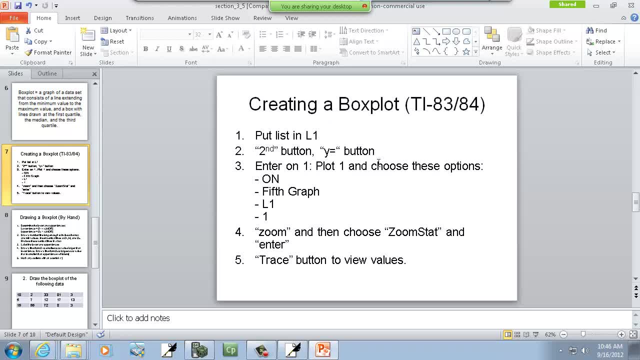 Then second button Y equals Enter on one plot one. Choose these options On the fifth graph, L1, 1. Zoom, then choose zoom stat and enter. Then trace to view the files Or view the values. sorry. 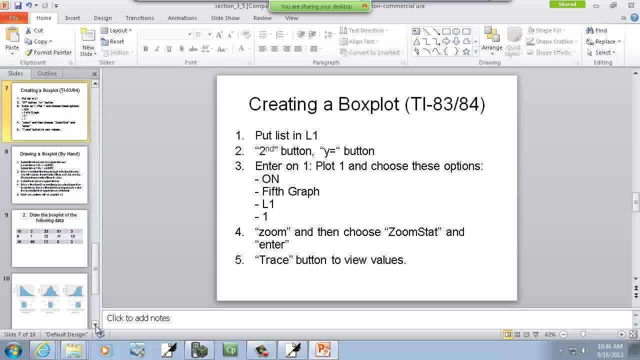 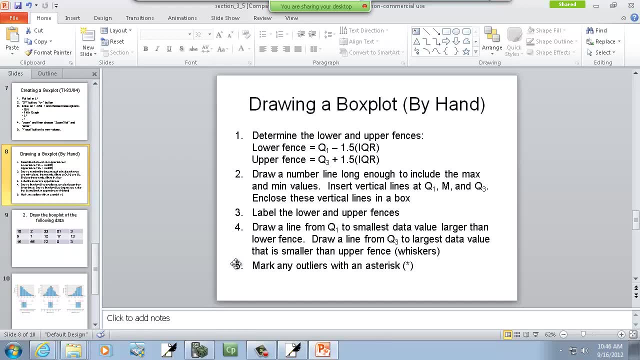 Now we'll show this with some data, So we'll come back to this Now. this is the draft. These are the directions that are in our current text book, And I don't really like these very well. It says: determine lower and upper fences. 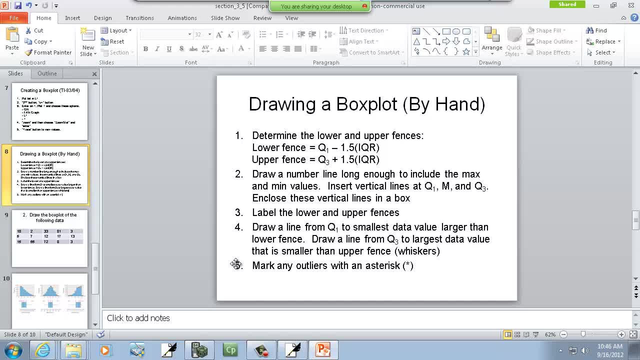 And that's just our typical formula. Lower fence is Q1 minus 1.5 times IQR, And upper fence is Q3 plus 1.5 times IQR And IQR is Q3 minus Q1.. Then it says: draw a number line long enough to include the max and min values. 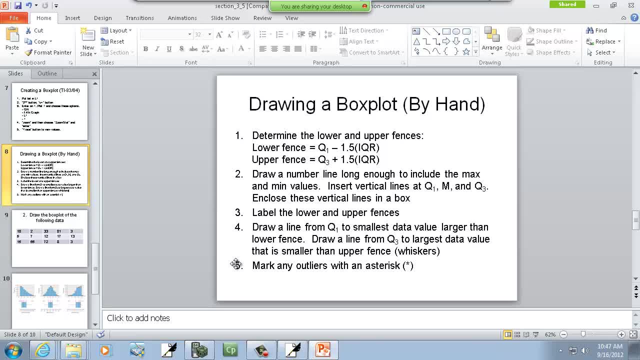 Insert vertical lines at Q1,, M and Q3. And close these vertical lines And a box, Label the lower and upper fences And draw a line from Q1 to your smallest data value larger than the lower fence. Draw a line from Q3 to your largest data value, the smaller than the upper fence. 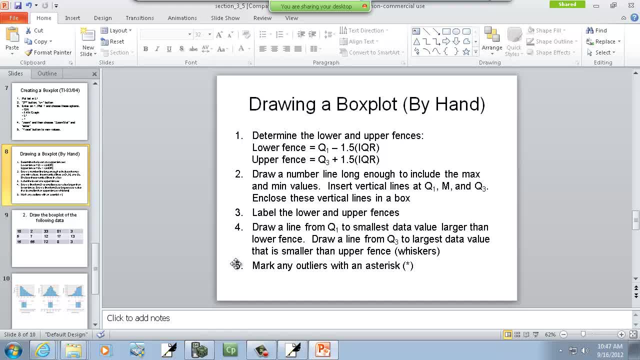 And these are referred to your whiskers Mark any outliers with an asterisk. My personal belief on this is that if you have an outlier, you should kick it out before you draw the box plot, And let me show you the reason why. 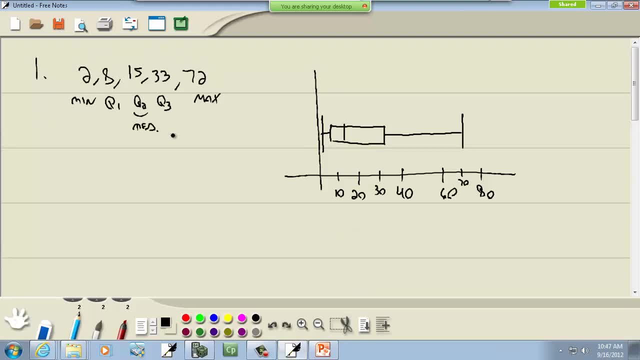 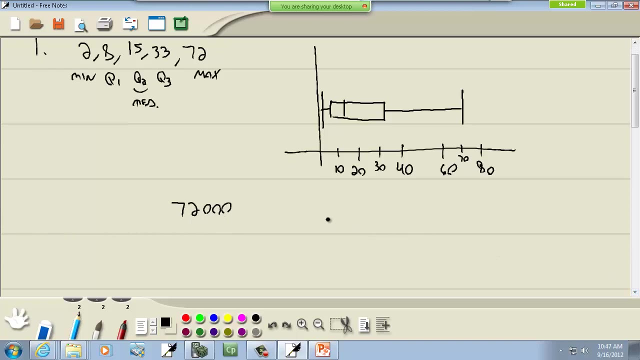 If I had these data points here, if, instead of 72, somebody had mistyped something and put in 72,000, well, if I came over here, here's 72,000, and this is where one of my data points is whether I put the max here or not. it indicates that I have 72,000 data points. 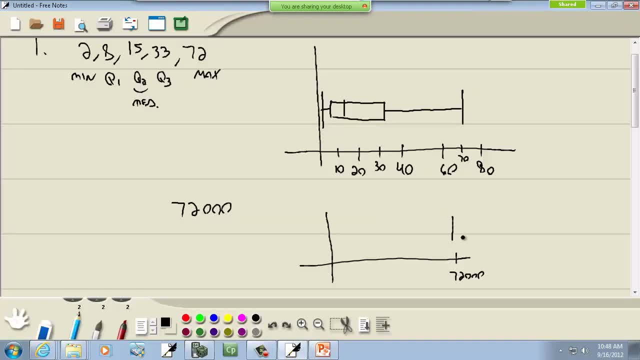 Okay, It indicates put an asterisk for the outlier. But you know, even actually let me go ahead and put an asterisk for the outlier. So here's my asterisk for my outlier: By putting 72,000 on there, what my box plot would look like is maybe that, right there. 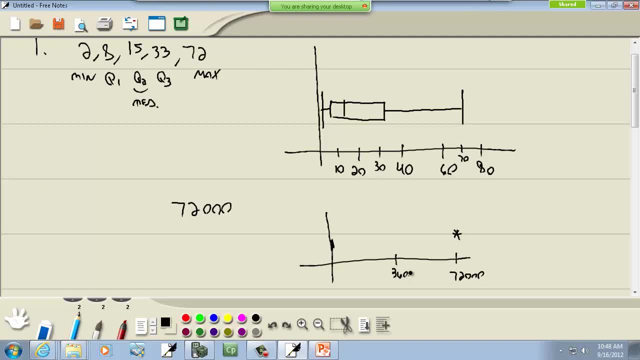 It wouldn't look like anything, Because you know here's 36,000.. You know here's 18,000.. So 72 would just be that little blip right there. So it really just messes the entire. 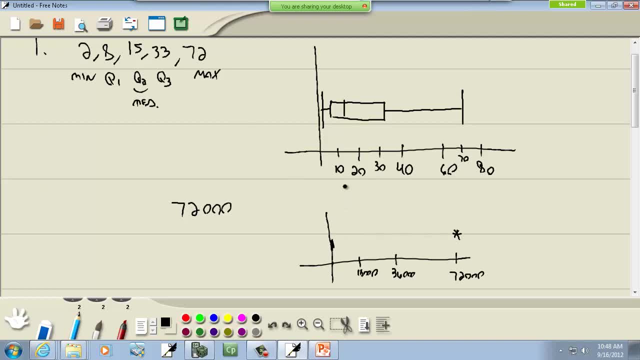 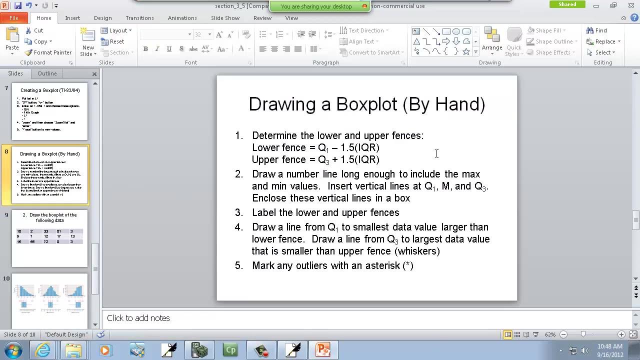 Thing up, Even if we exclude that. So my personal belief is: take out the outliers before you draw the box, plot, You know, find your IQR, your fences and so forth, and remove those. Well, but I wanted to give you that, since that was in our current textbook. 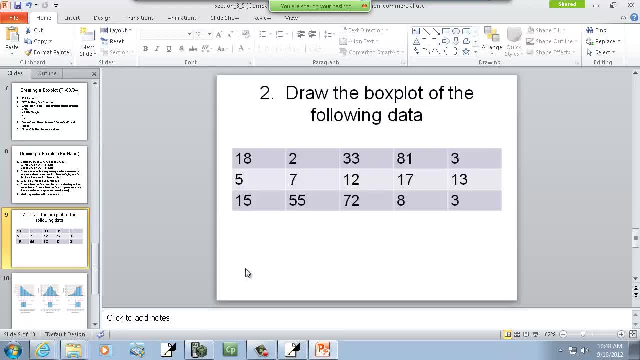 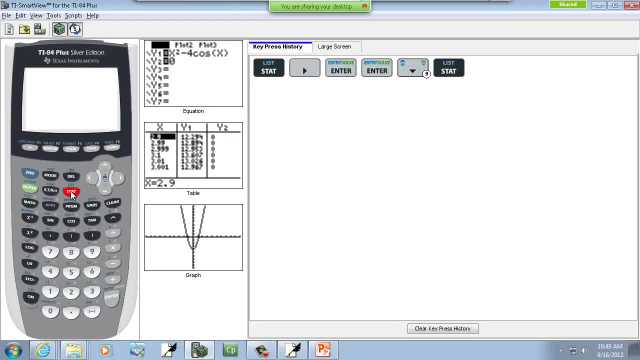 It's much better to do what I did in the example above. Well, let's draw one using the calculator now. So I'm going to need to input these numbers, So I'll press- I'm going to do this quick way now and press clear. 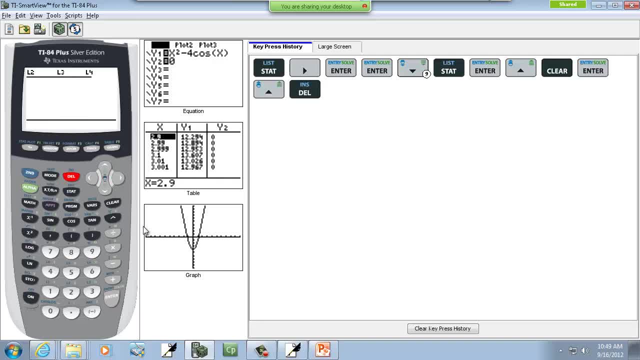 Now, if you up arrow and again press delete, by accident your L1 is gone. Well, what you do is if you could come back in here. you notice L1 is gone. If you up arrow and highlight L2, you do second delete to go into insert. 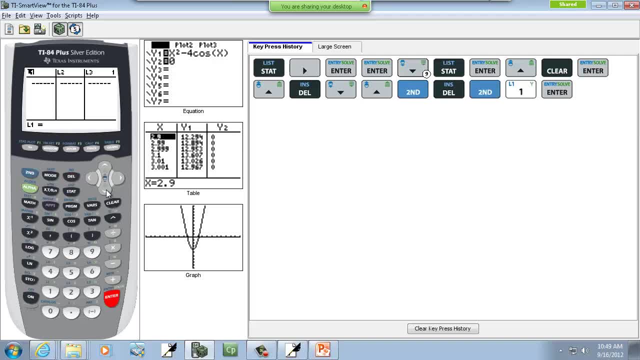 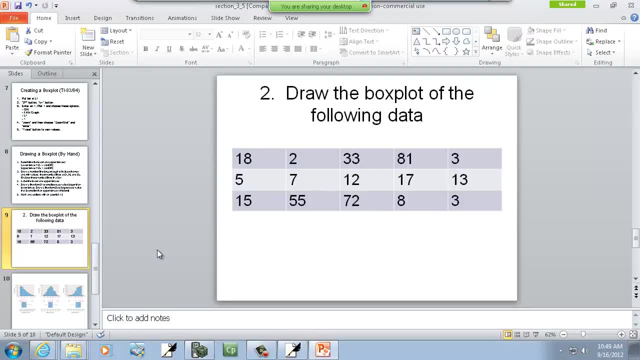 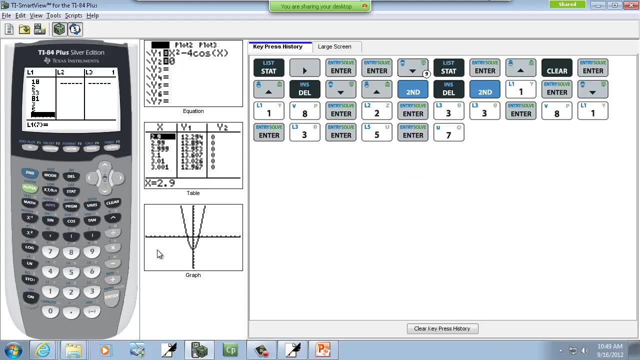 And then do second one enter, And that will put L1 back. Okay, So let's put our numbers in: 18 enter 2. enter 33. enter 81. enter 3. enter 5. enter 7 enter. 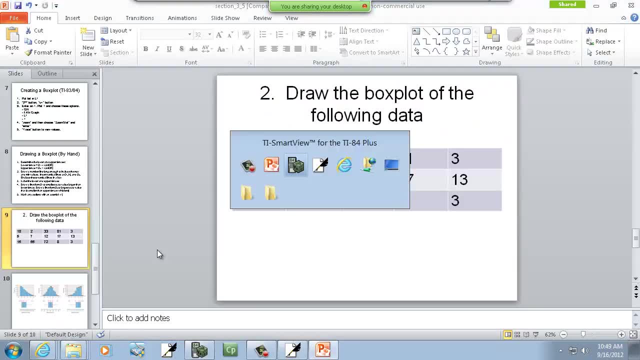 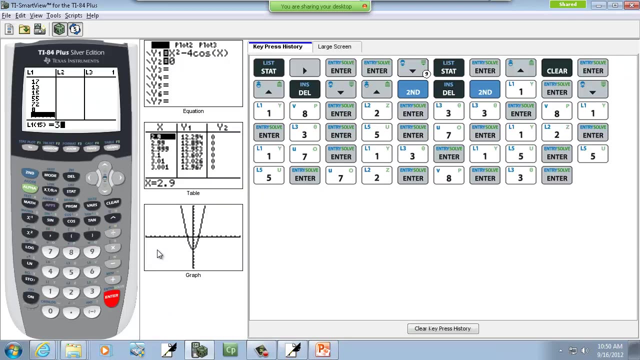 12 enter 17 enter. 13 enter. 15 enter. 55 enter. 72 enter. 72 enter. 8 enter. 3 enter. I'm going to double check my numbers. I'm not very good at data entry. 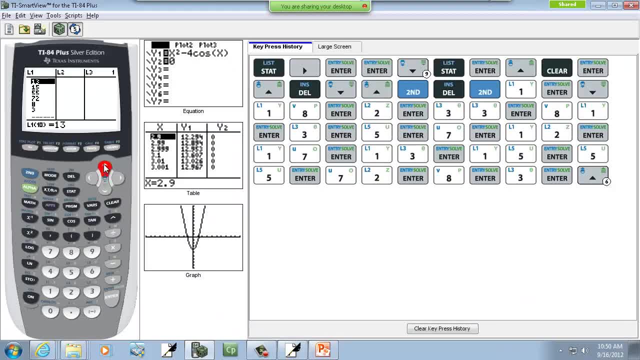 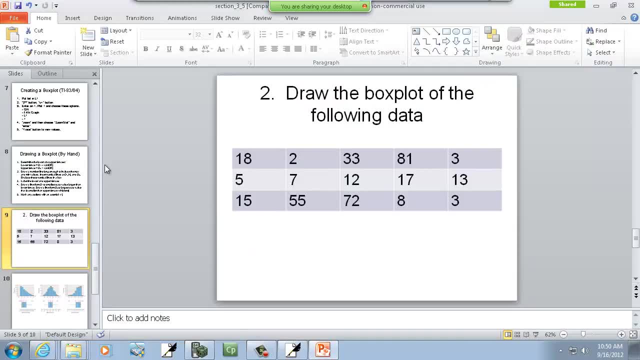 3,, 8,, 72,, 55,, 15,, 13,, 17,, 12,, 7,, 5,, 3,, 81,, 33,, 2, and 18.. Okay, Okay. So now let's second mode. 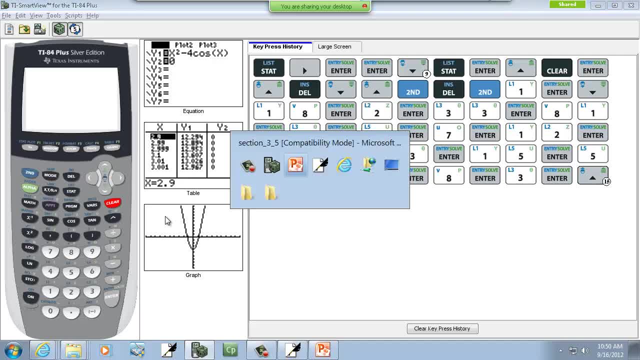 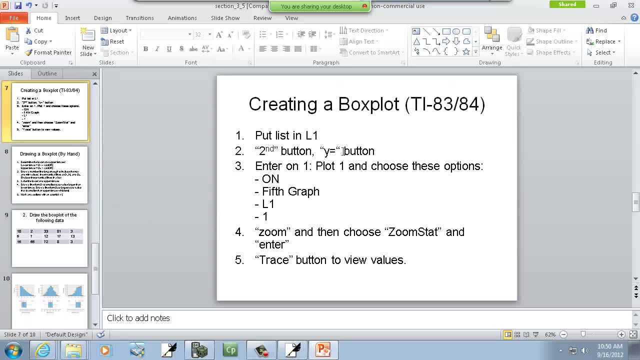 We're going to fix it out, Okay, So I'm going to go back up here. Put your list in L1.. We just did that. Then it says do a second, y equals. So we'll press. let me get rid of those. 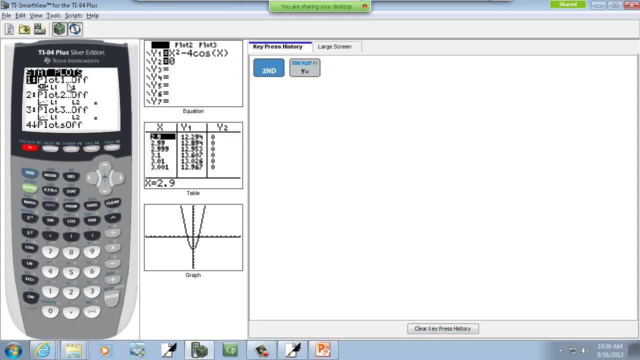 Second, y equals. Now I notice, plot one is already highlighted. It says: enter on one plot one, Then choose these options. We want the graphs as on. So let's do that, Let's do that, Let's do that. 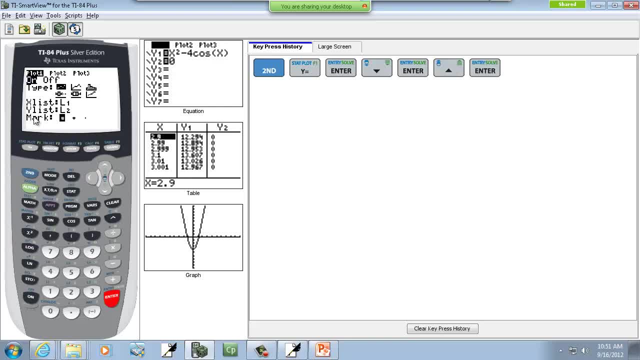 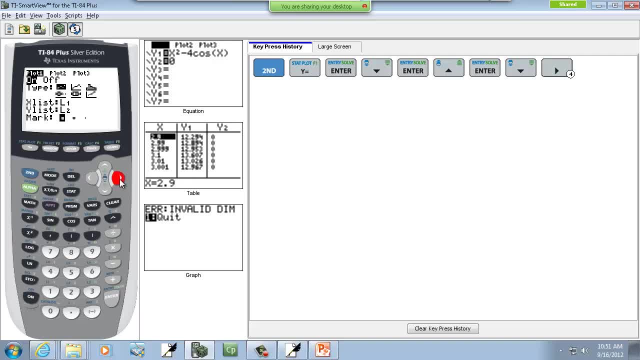 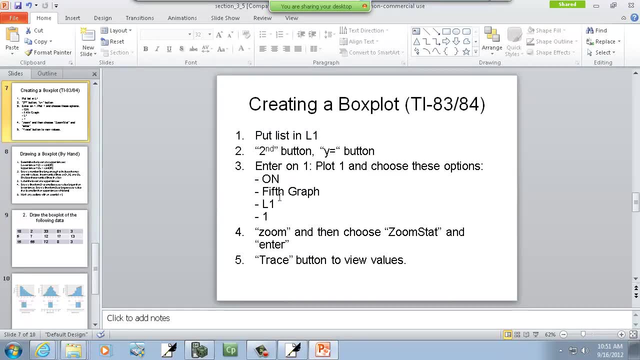 So I have to use my right arrow to go to it. Don't use your down arrow, And it's not hard. You pick the one that looks like a box plot, Then press enter on it, And then it defaults to L1 and 1, which I'm happy with. 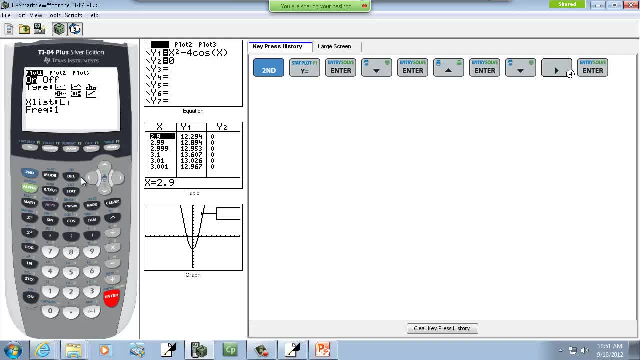 So you can leave those as is Now. you shouldn't have to do this, but I did some trig earlier in my calculator So I'm going to have to go to y equals And clear out y1.. 0 and y2 doesn't hurt anything. 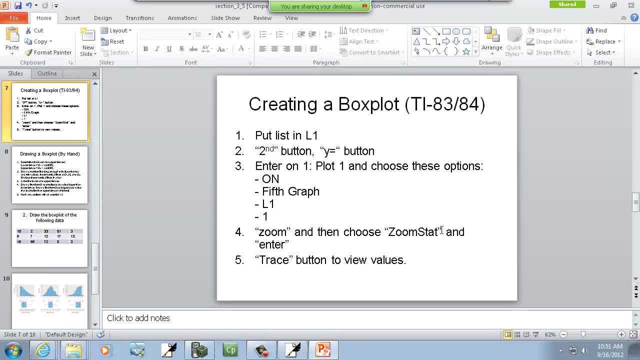 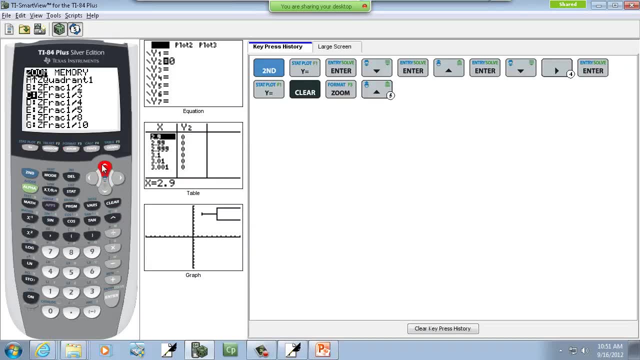 And then this tells us to choose zoom and then choose zoom stat. So I'll press zoom And I want to up arrow. I have a lot of other options, but you shouldn't have that many, Unless you've got one of the older T84s. 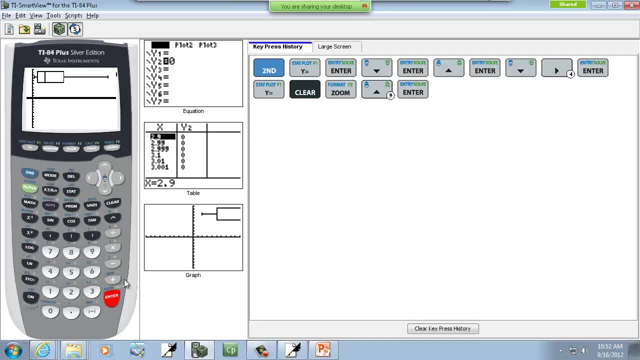 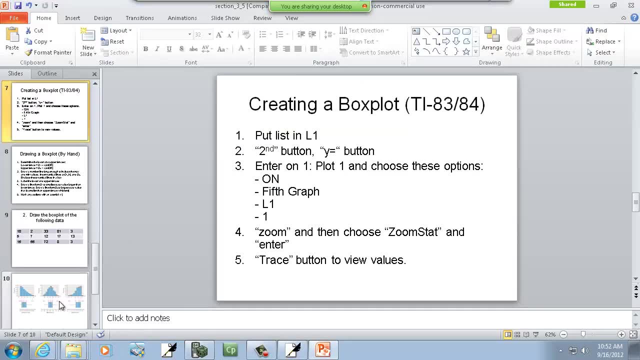 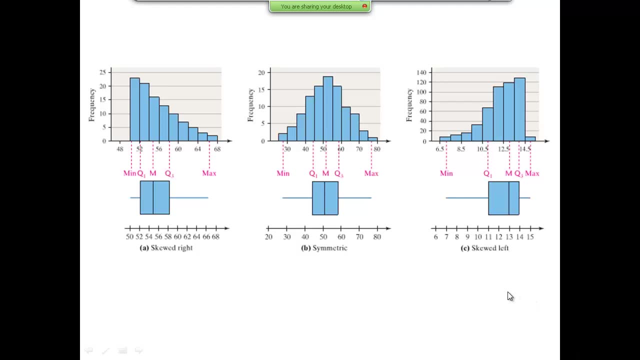 We want to choose zoom stat And now give us our box plot. OK, what can we use a box plot for? Let me make this a little bit bigger so we can see it. This is one method to allow you to see if your data is skewed. 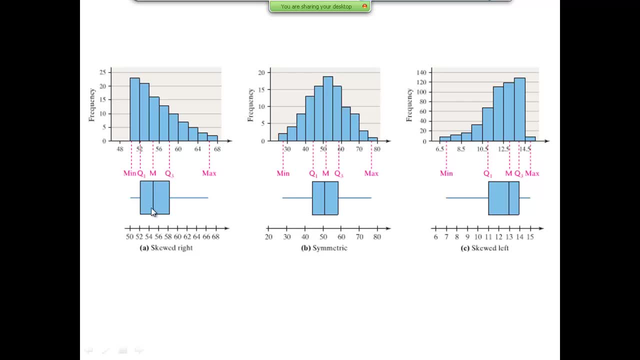 If it's skewed left, skewed right, or if it's symmetric. Now again, this is kind of opposite of what you think, If you look at this first graph here, where all of your data looks like it's over on the left side. 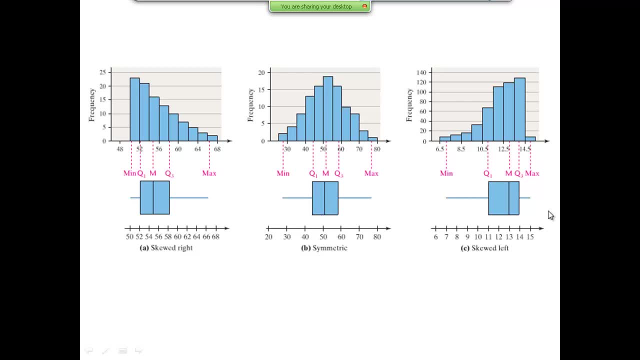 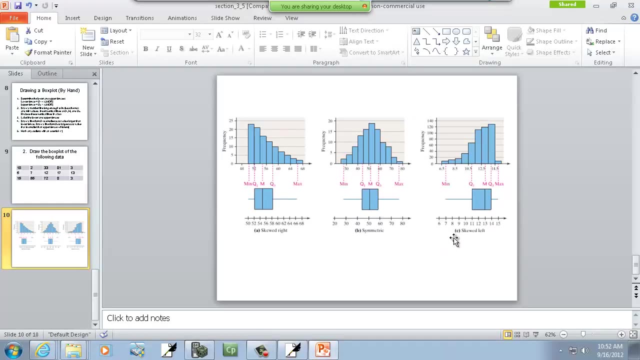 that's skewed right. If it's roughly in the middle, it's symmetric, And then if your data appears, it's skewed right. If it appears to be over here on the right side, then it's skewed left. So for this one, see how all of our data looks like it's on the left side. 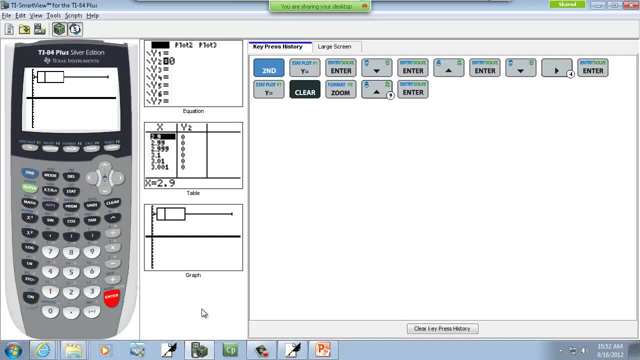 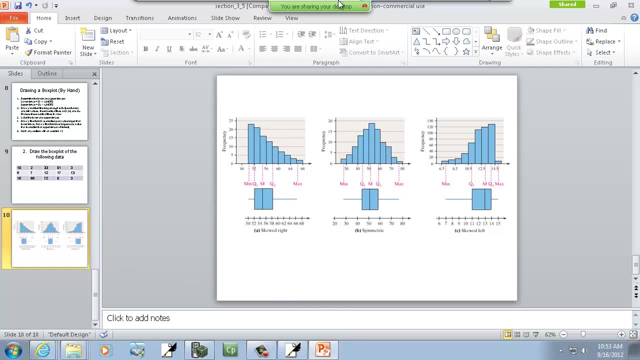 So this is skewed right. So it's a very easy way to determine that You don't have to draw your bar graphs and see how things are arranged- Very quick way to do it. And that's the last of that section, So let me stop the recorders here.